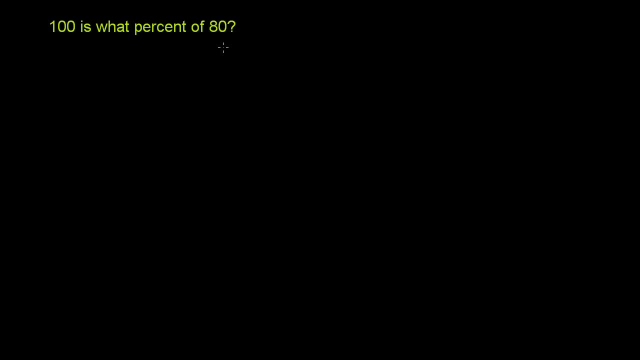 100 is what percent of 80?? And these problems tend to kill people because on some level they're kind of simple: There's just 100 and an 80 there and they're asking what percent. but then people get confused. 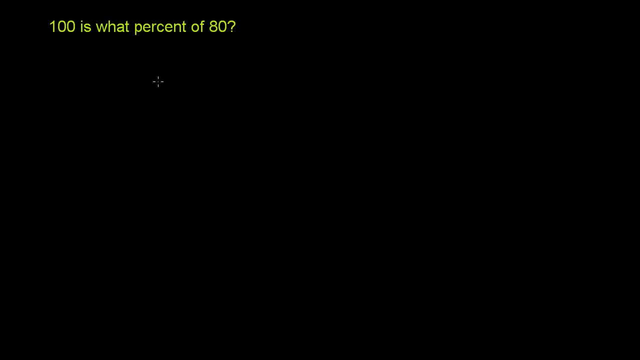 They say: do I divide the 100 by the 80,, the 80 by 100, or is it something else going on And you really just have to think through what the language is saying. They're saying that this value right here, this 100, is some. 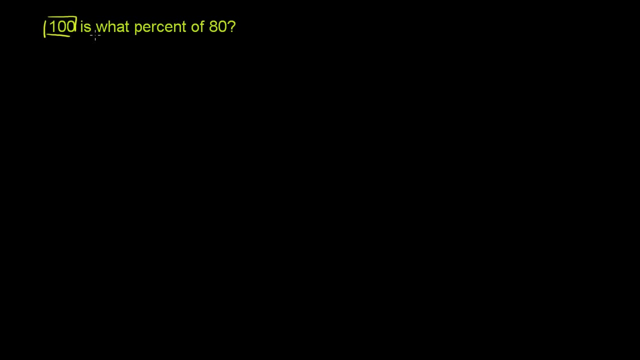 percentage of 80, and that some percentage is what we have to figure out. that what percent? So if we multiply 80 by this, what percent? we will get 100.. So let's view it this way: We start, we have 80.. 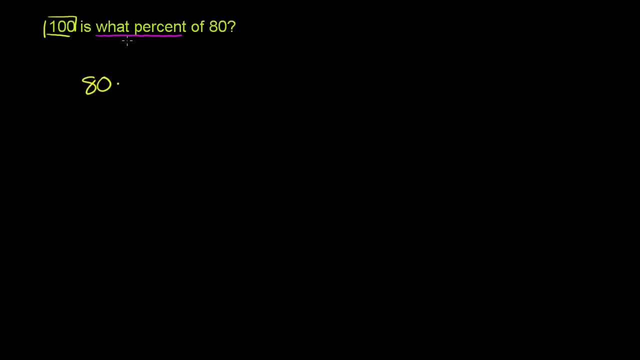 If we multiply it by something, let's call this something x. If we multiply, let me do that in a different color. If we multiply 80 by something, we're going to get 100. And we need to figure out what we need to multiply 80 by to. 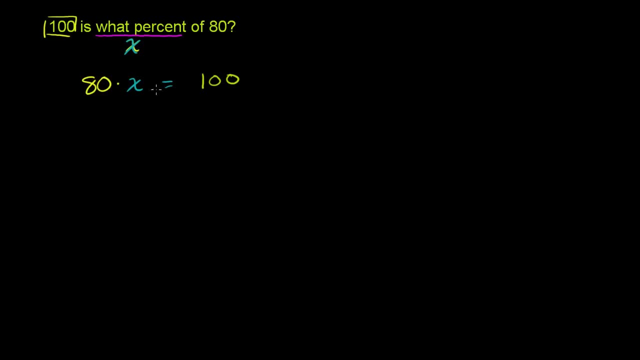 get 100.. And if we just solve this equation as it is, we're going to get a value for x and what we need to do is then convert it to a percent. Another way you could view this is: 100 is what you get. 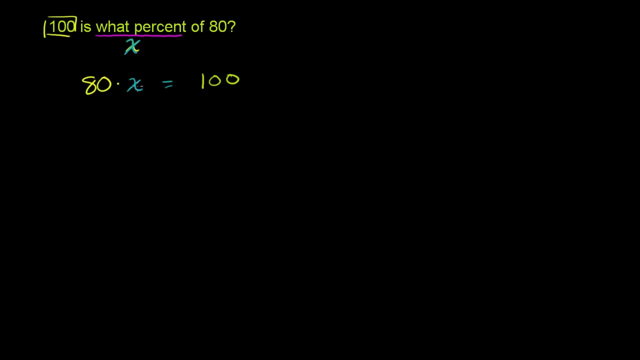 when you multiply what by 80. And then you would have gotten this number and then you could convert it to a percent. So this is essentially the equation. and now we can solve it If we divide both sides of this equation by 80, so you: 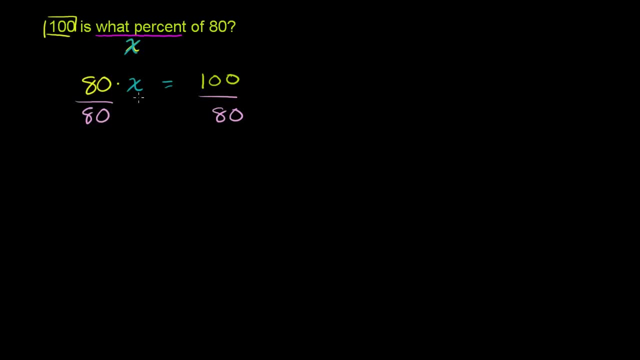 divide the left-hand side by 80, the right-hand side by 80, you get x. x is equal to 100 over 80. They both share a common factor of 20, so 100 divided by 20 is 5, and 80 divided by 20 is 4.. 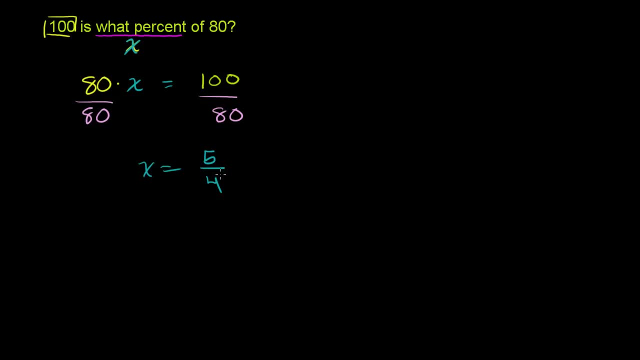 So in simplest form, x is equal to 5 fourths, but I've only expressed it as a fraction. But they want to know what percent of 80.. If they just said 100 is what fraction of 80, we would be. 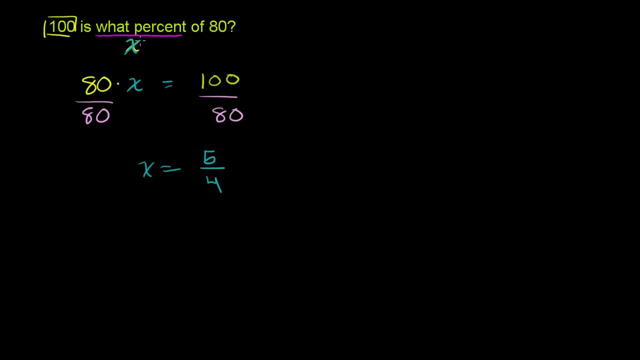 done. We could say 100 is what percent of 80.. We could say 100 is what fraction of 80.. We could say 100 is 5 fourths of 80, and we would be absolutely correct. But they want to say what percent. 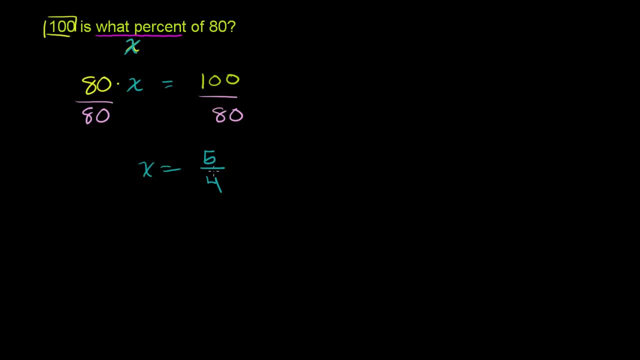 So we have to convert this to a percent, and the easiest thing to do is to first convert it into a decimal. So let's do that. 5 over 4 is literally the same thing as 5 divided by 4.. So let's figure out what that is. 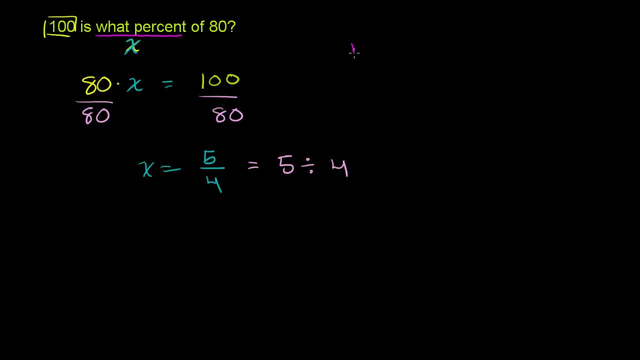 Let me do it in magenta. So 5 divided by 4.. 5 divided by 4, and we want to have all the decimals there, So let's put some 0's out here. 4 goes into 5 one time. 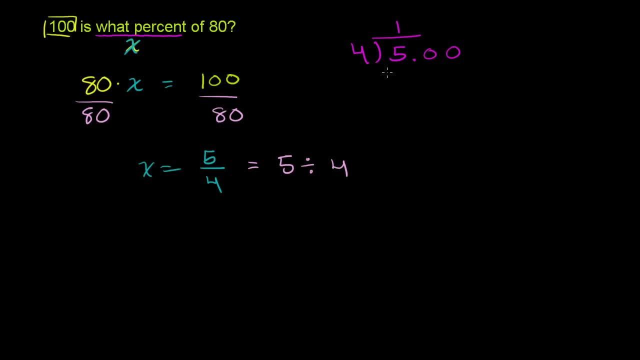 Let me switch up the colors One time: 1 times 4 is 4.. You subtract, You get 5 minus 4 is 1.. Bring down the next 0. And of course the decimal is sitting right here. so we want. 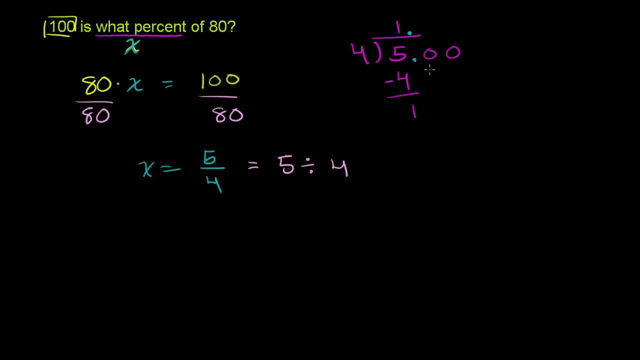 to put it right over there. So you bring down the next 0.. 4 goes into 10. two times 2 times 4 is 8.. You subtract 10 minus 8 is 2.. Bring down the next 0.. 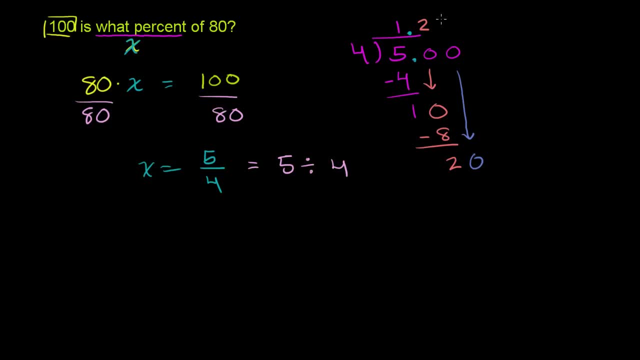 Bring down the next 0.. 4 goes into 20. five times 5 times 4 is 20.. Subtract No remainder, So this is exactly equal to 1.25.. 5 over 4 is the same thing as 5 divided by 4, which is equal. 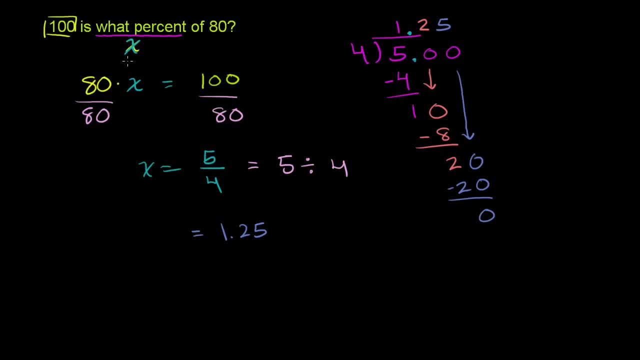 to 1.25.. So so far we could say 100 is 1.25 times 80. Or 1.25 of 80, you could even say it, But we still haven't expressed it as a percentage. This is really just as a number. 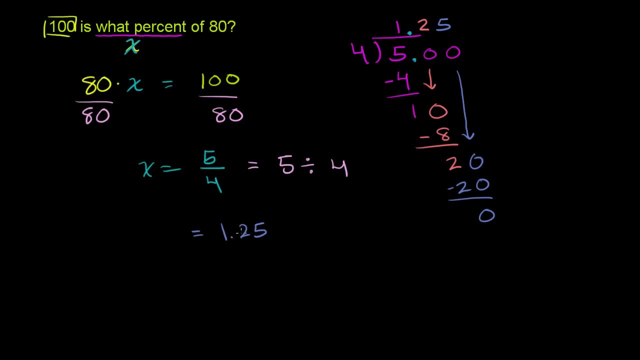 I guess you could call it as a decimal, But it's a whole number and a decimal. It would be a mixed number if we didn't do it as a decimal. It's 1 and 1 fourth, or 1 and 25 hundredths. 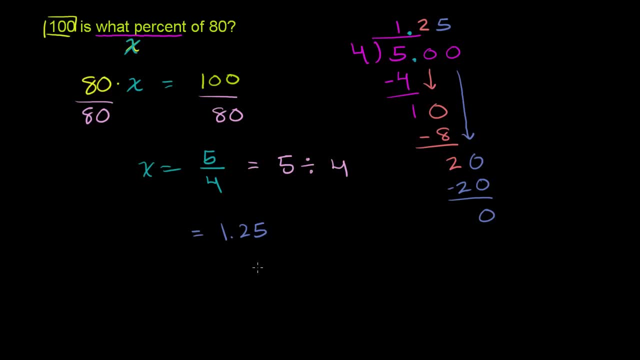 however you want to read it. So to write it as a percent, you literally just have to multiply this times 100, or shift the decimal over twice. So this is going to be 1.25.. This is going to be equal to as a percent.